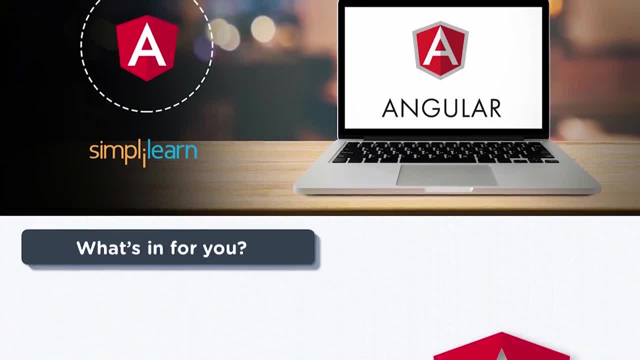 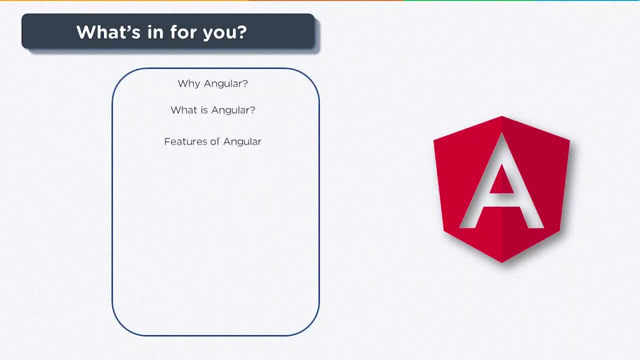 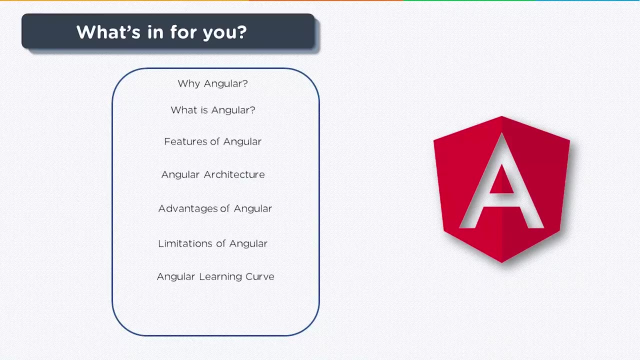 dive into the session now. So here is a list of topics that we're going to be covering. First up, we'll see why Angular was introduced, Then what is Angular, features of Angular, Angular architecture and how Angular works, And finally, we'll look at some of the companies that deploy Angular. So, without further delay, 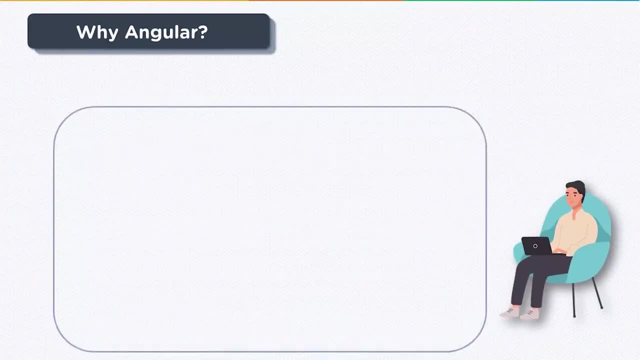 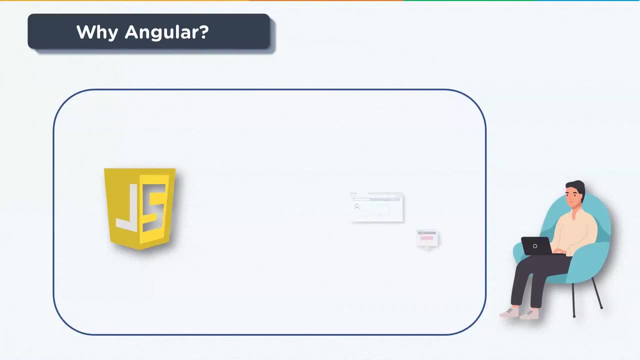 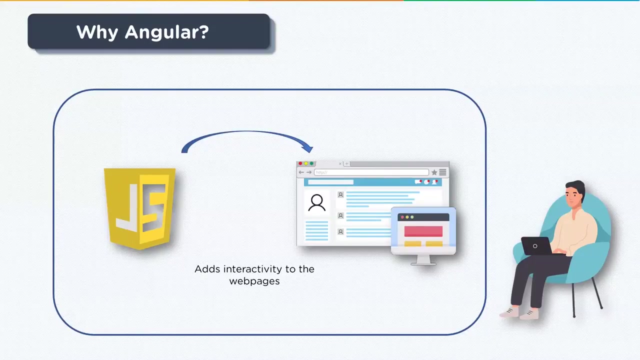 let's begin. Why Angular Now? JavaScript is the most commonly used client-side scripting language. It is written into HTML documents, enabling interactions with web pages in many unique ways. So, as a relatively easy-to-learn language with almost pervasive features, it's easy to learn languages. 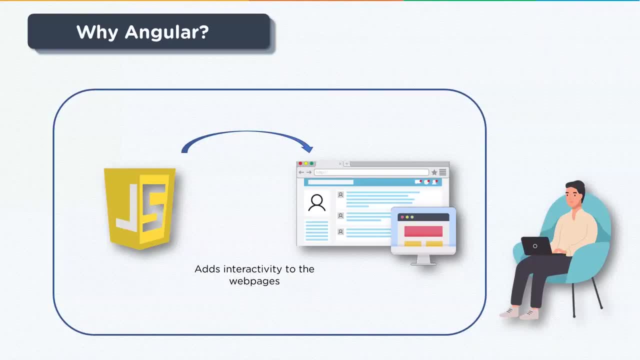 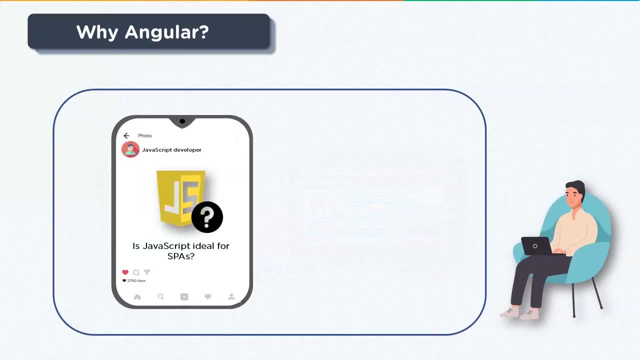 and you can use it to develop your own apps. However, in terms of language, it's not the most pervasive support. It is exceptionally well-suited to develop modern applications, But the question arises: Is JavaScript ideal for developing single-page applications that require modularity, testability and other? 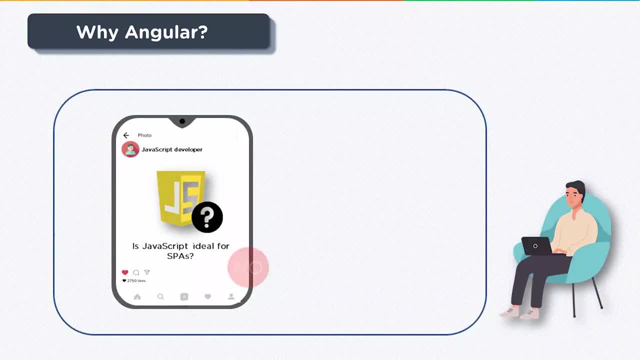 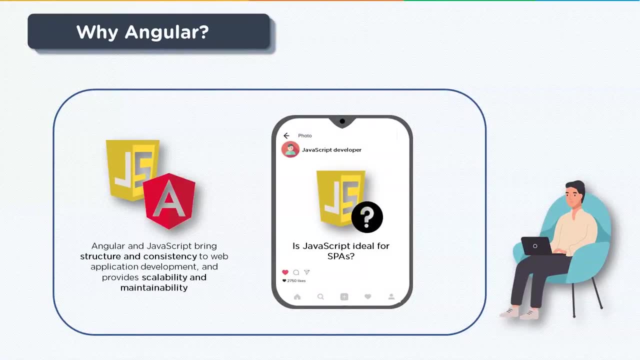 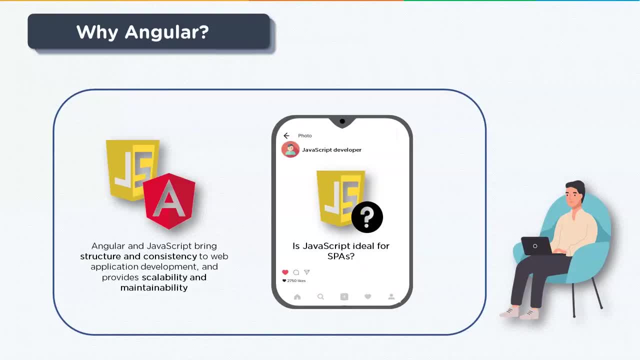 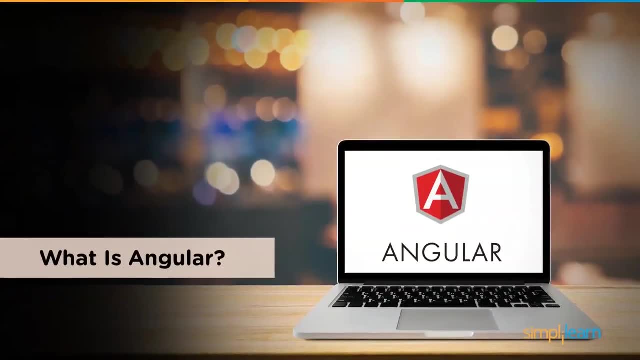 get started. So let's get started, Let's get started. And also it provides scalability and maintainability. Angular is specifically developed for single-page applications. Now the question arises: What exactly is Angular? Angular is an open-source JavaScript framework. 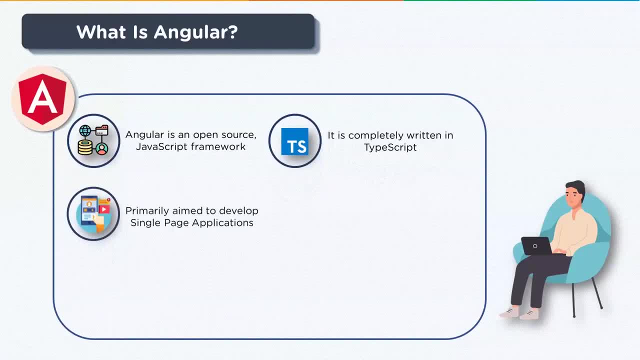 written completely in TypeScript Now. it was primarily aimed to develop single-page applications and is maintained by Google. Angular as a framework provides a few advantages while also providing a standard structure for developing single-page applications, And it's also esfuercing to develop and maintain those single-page apps. So let's get started. 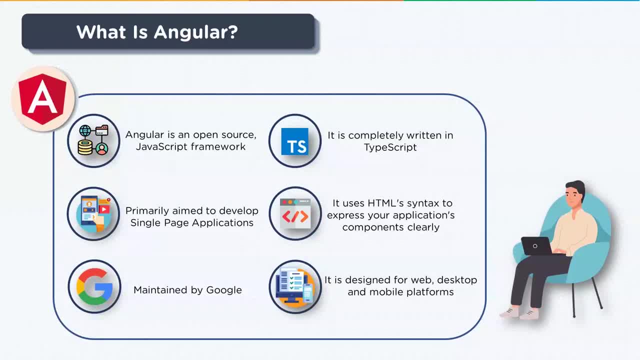 Now the first one, So let's start with the first one. So let's start with the first one. Or developers? It is designed for web, desktop and mobile platforms. If you have a doubt here as to what exactly single page applications are, let me help. 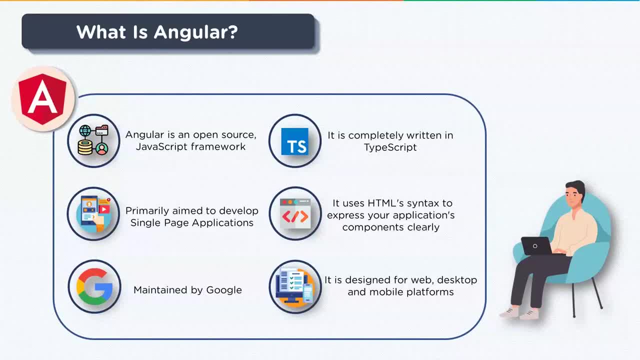 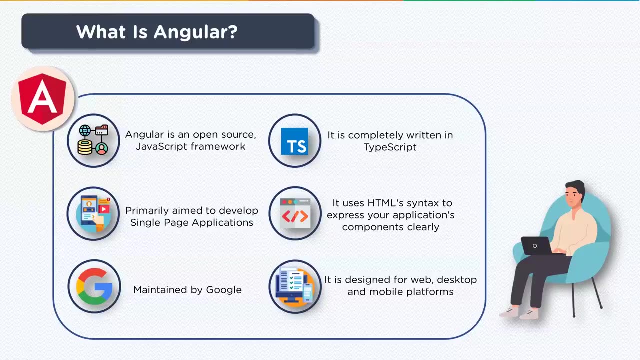 you with that. Now, these single page applications are basically applications that get loaded just once, So the main page gets loaded onto your browser, So any further interactions does not lead to loading of subsequent pages. Anything that has to be done further is just an addition to the already loaded page. These single-page applications are primarily developed. 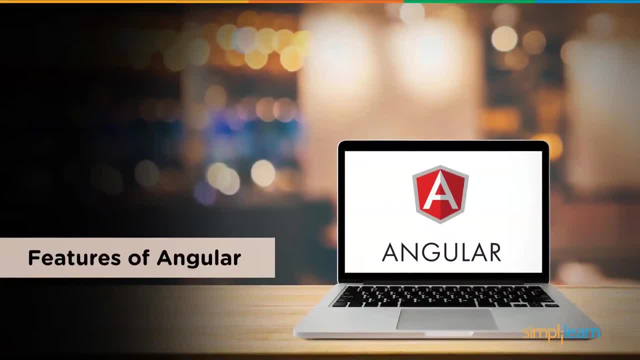 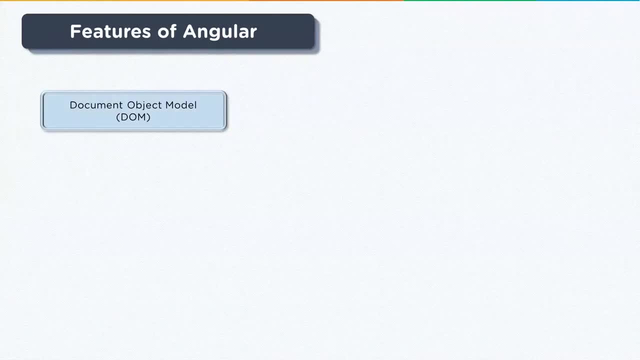 using Angular. Moving ahead, let's look at the features of Angular. We have four features that we're going to be discussing. We have the document, object, model, tag, script, data binding and testing. Now let's look at them one by one. 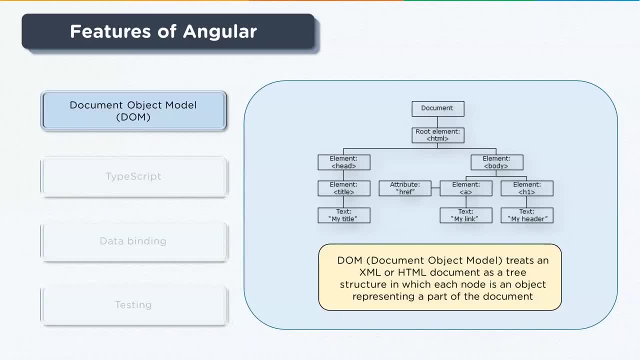 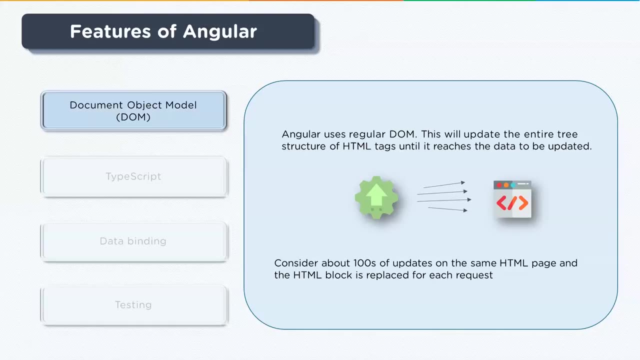 Now the document object model treats an XML or an HTML document as a tree structure. Now, here in the tree structure defines an object representing a part of your document. Angular uses the regular DOM. Now, let's suppose you've made 10 updates on a. 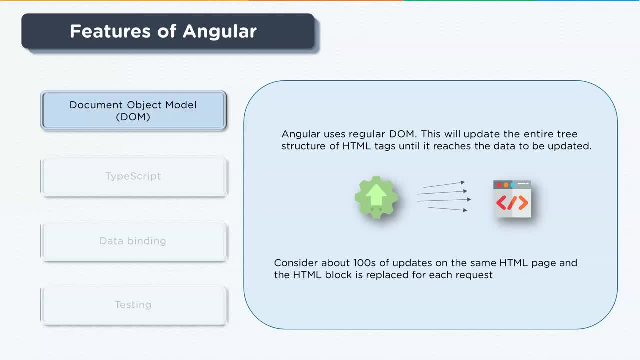 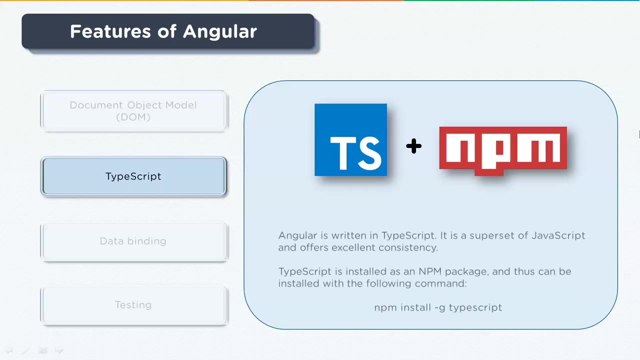 single HTML page. So every time you make a change, the corresponding DOM or the tree structure needs to be updated. Now Angular updates the entire tree structure of HTML tags. Moving on to our next feature, we have TypeScript. Now TypeScript defines a set of types to JavaScript, which helps you write. 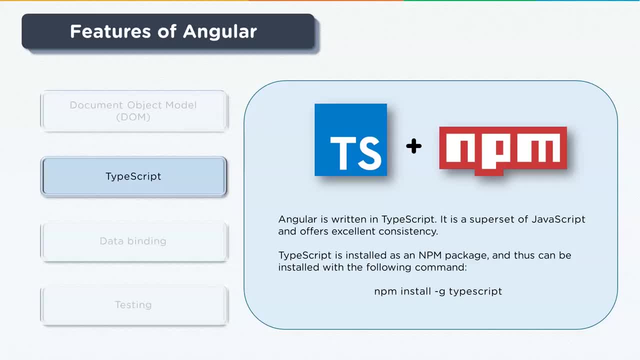 JavaScript that is easier to understand. Now all the TypeScript code compiles down to basic JavaScript that can run smoothly on any platform. Now TypeScript is not mandatory for developing an Angular application, but it is highly recommended. The main reason it's highly recommended is that it offers better. 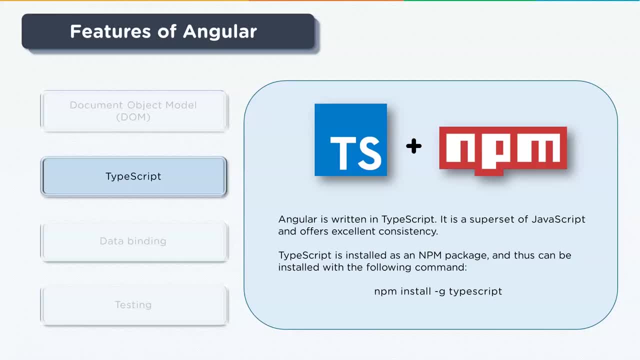 syntactic structure while making the code base easier to understand and maintain. now types: you can be installed as an npm package. now, to do that, you just have to run the command npm install hyphen g typescript on your command prompt. next up is data binding. now data. 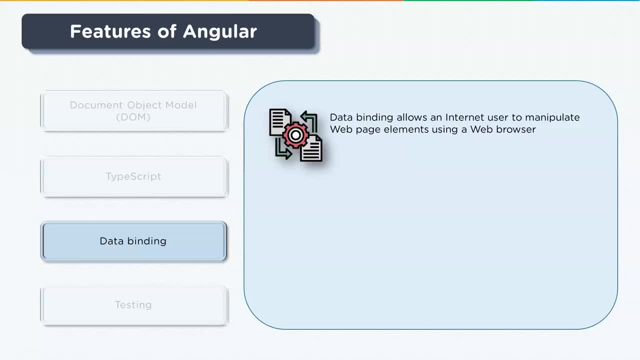 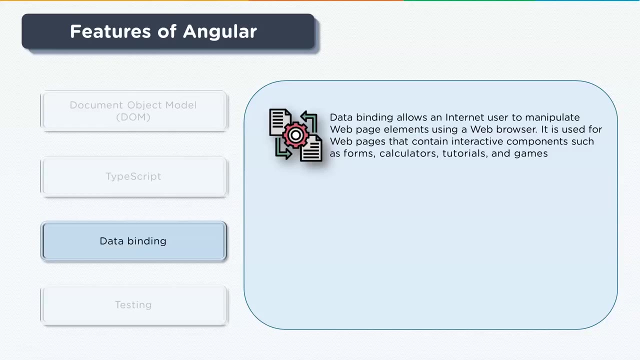 binding is a process that allows you to manipulate web page elements using the web browser. now it mainly employs dynamic html and does not require complex scripting or programming. it is used in web pages that include interactive components like calculators, tutorials, games, etc. now, incremental display of a web page makes data binding extremely convenient when pages contain a large amount of. 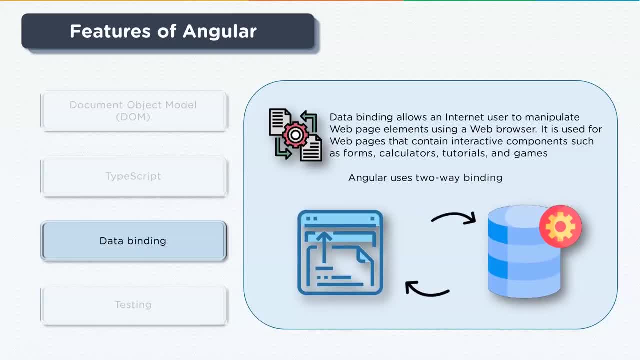 data. when it comes to angular, it uses two-way data binding, so any changes made in the ui element is reflected in the corresponding model state and, conversely, any changes made in the model state are reflected on two-way data binding in the web pages. now data binding is extremely convenient. 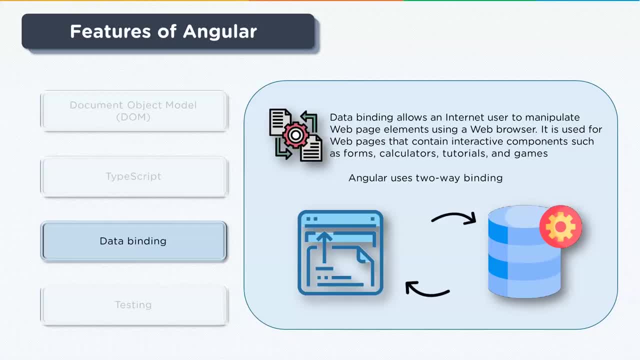 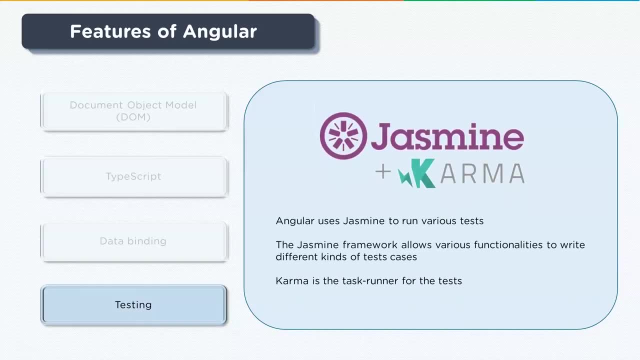 the UI state. This allows the framework to connect the tom to the model data via the controller. The last feature we're discussing is testing. Angular uses Jasmine to run its various tests. The Jasmine framework allows various functionalities to write different kinds of test cases. Karma is a task runner for the tests that use a configuration file to set the startup. 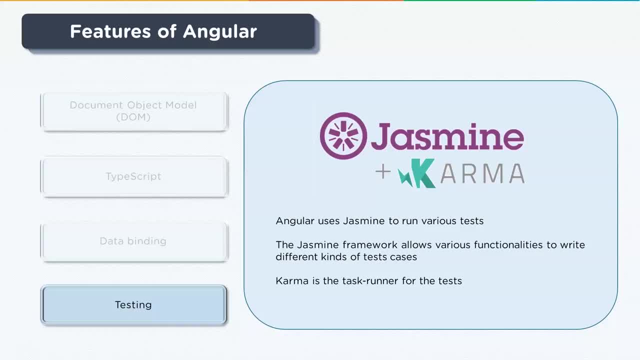 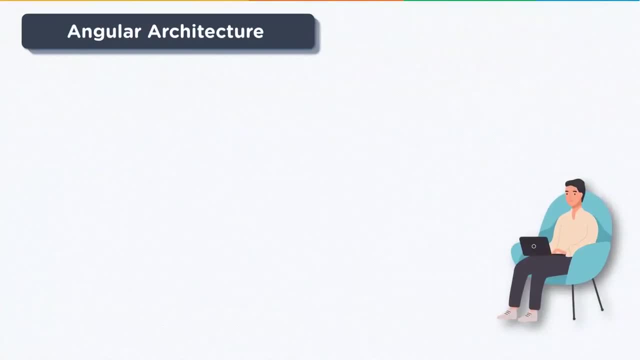 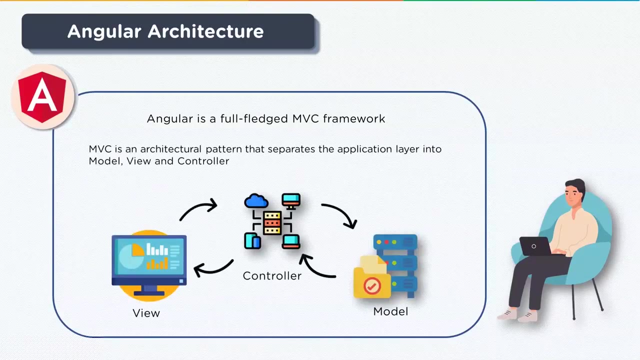 reporters and testing framework. So with that, we've covered the features of Angular. So let's go ahead and understand the architecture of Angular Now. Angular is a full-fledged MVC framework. It provides a strong opinion on how the application should be structured. 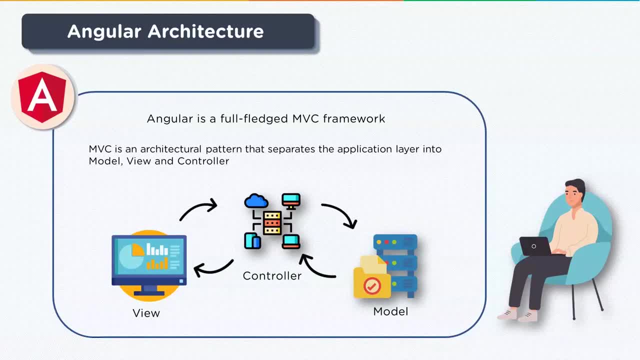 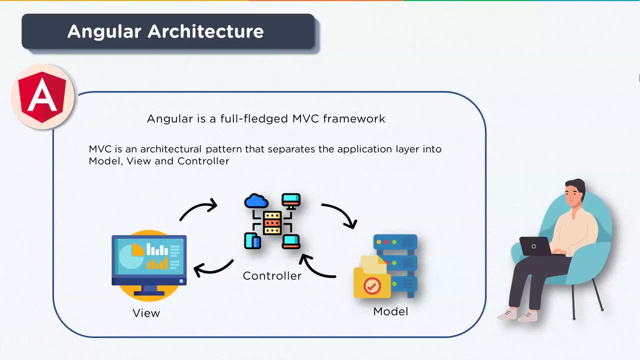 and offers bi-directional data flow and updates. the real DOM MVC- short for Model View Controller- is an architectural pattern that separates the architecture from the model. Now, if you have a model and you want to get the actual application layer into model view and controller, model here relates to all the data related logic. 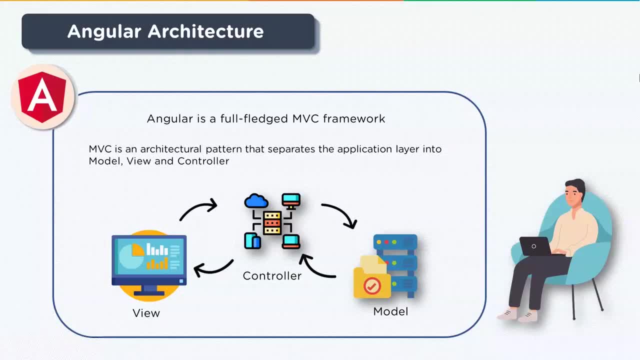 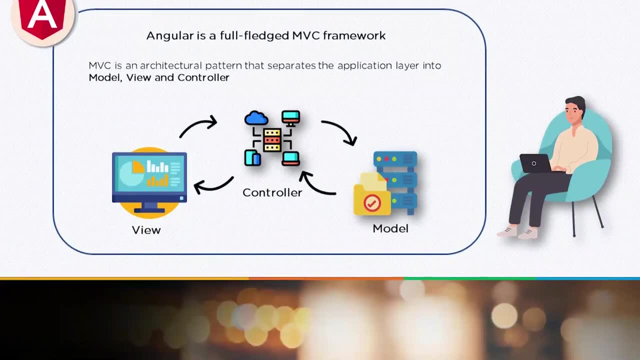 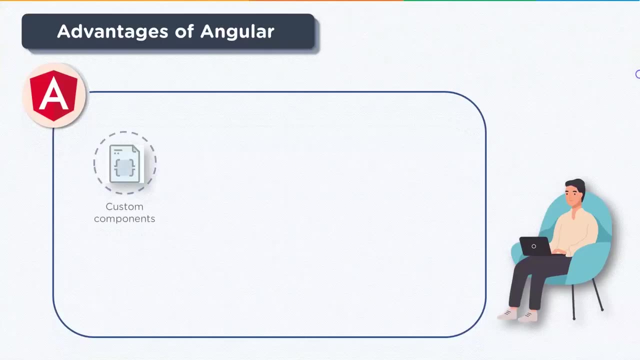 view, on the other hand, is used for ui logic of the application, and controller is the brain of the setup. now it is an interface between the model and view. moving on, let's look at the advantages of angular. first up, we have custom components. angular allows you to. 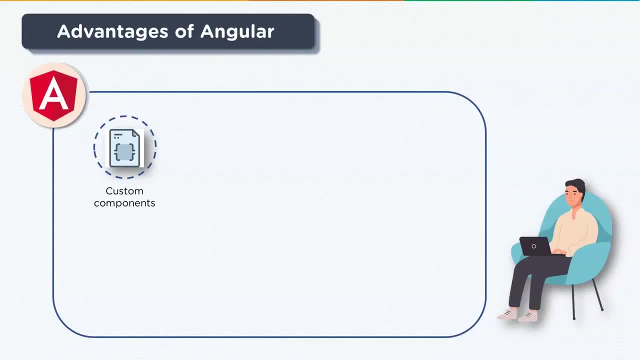 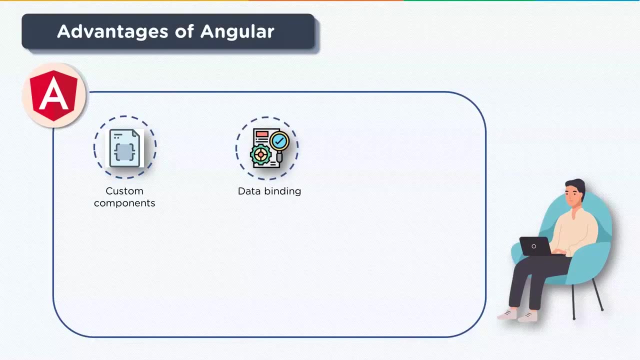 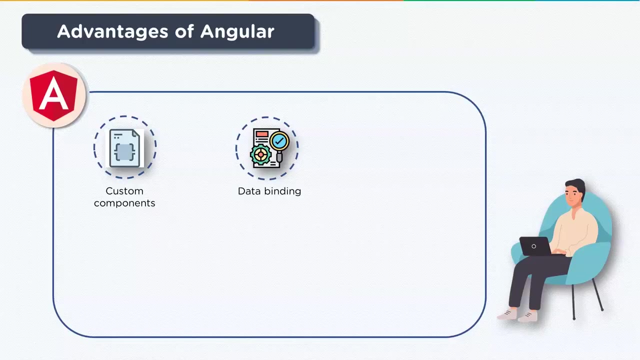 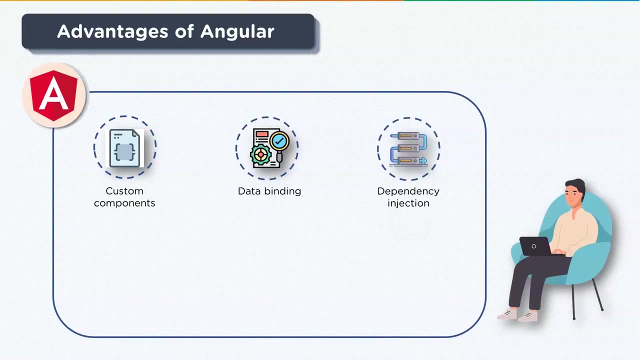 build your own components that can pack functionality along with rendering logic into reusable pieces. data binding: as discussed, angular allows you to effortlessly move your data from your javascript code to the view and react to user events without having to write any code yourself. dependency injection angular allows you to write modular services and have them injected. 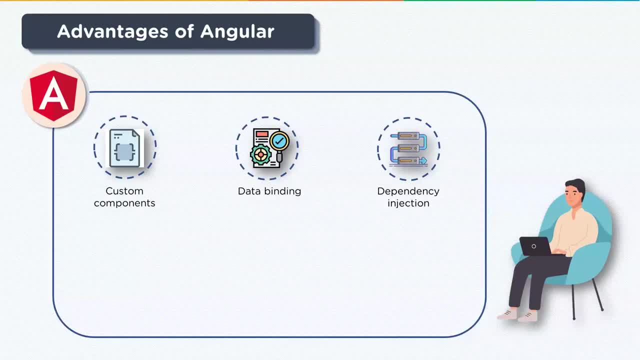 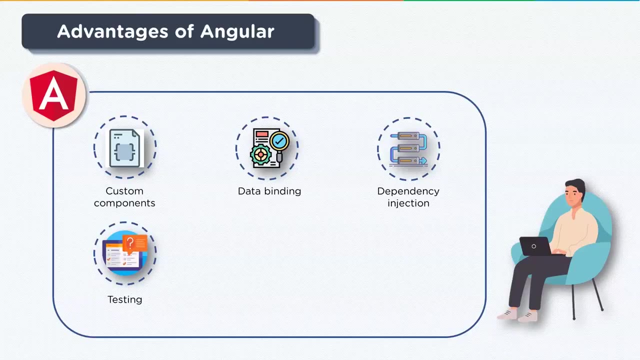 wherever they are needed. this greatly improves the testability and reusability of the same. don't worry if you can't wrap your head around these topics. we're going to discuss them further in the coming videos. next advantage is testing. angular has been built from the ground up with testability in mind. you 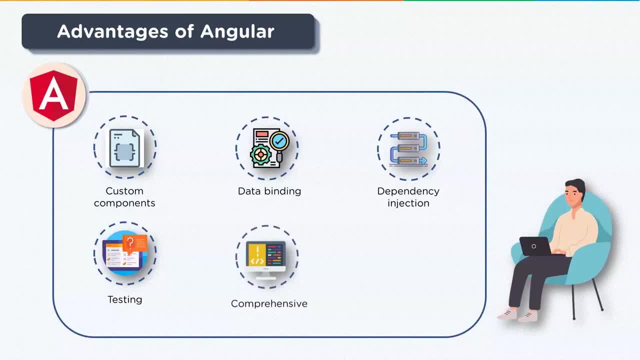 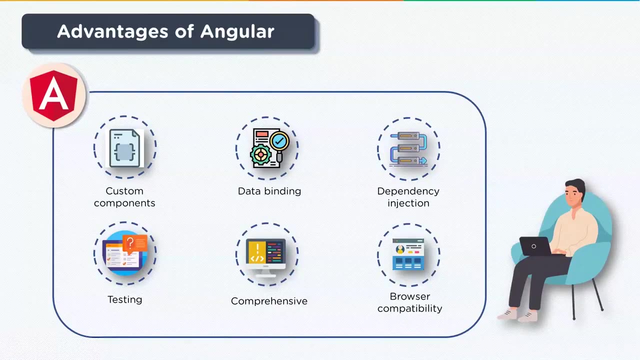 can literally test every part of your application. comprehensive angular is a full-fledged framework and provides out-of-the-box solutions for server communication, routing and mark. lastly, we have excellent browser compatibility. angular is cross-platform and browser compatible. an angular application can typically run on all browsers. 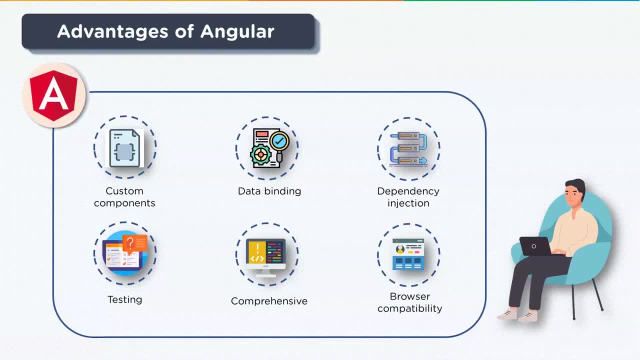 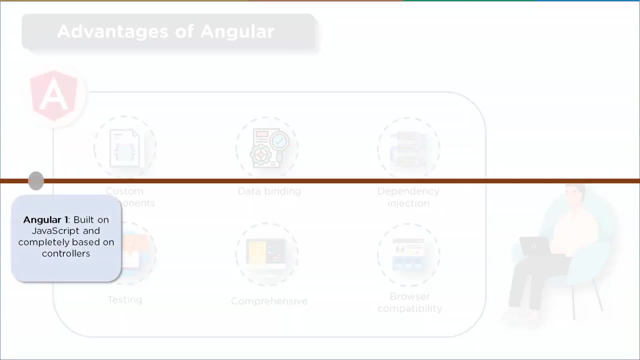 beat chrome, firefox, safari and platforms like windows, mac os and linux. now, many versions of angular have been released ever since its inception. all of these versions have added to the efficient working of the framework. now here are the different versions released. First up was Angular 1. It was built on JavaScript and completely based on controllers. 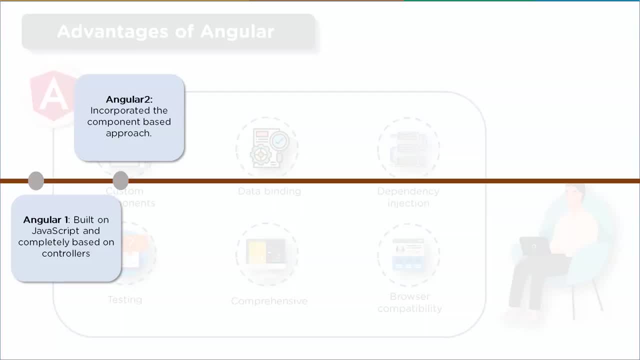 Next release was Angular 2.. Now this incorporated the component-based approach, wherein the entire UI was divided into several components and lastly integrated to give the final logic. Next was Angular 4.. It included router updation. Angular CLI or command line interface 1.0 was 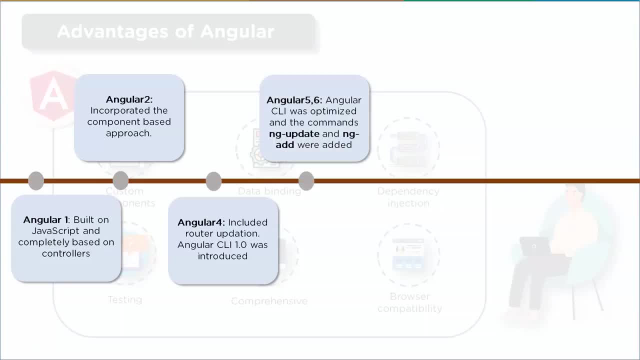 introduced, however not deployed In this release. the Angular CLI was optimized and commands like ng-update and ng-add were added. In the Angular 7 release, prompts were introduced which provided tips in CLI about the functions being used. In Angular 8, Ivy Renderer and Bazel were introduced. 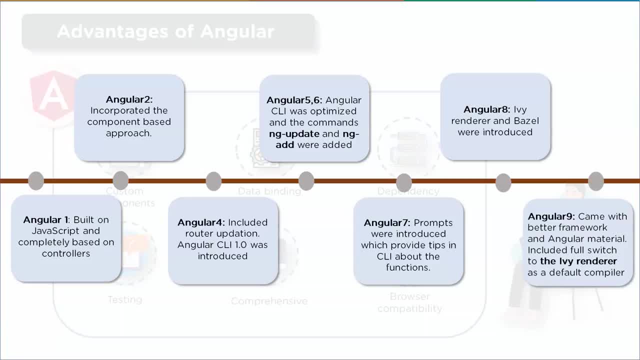 And finally, the most recent release was Angular 9.. Now this came with the better framework and Angular material. Now this completely switched to the Ivy Renderer as a default compiler. Now that we've learnt about the pros of using Angular, let's look at some of the limitations of Angular. 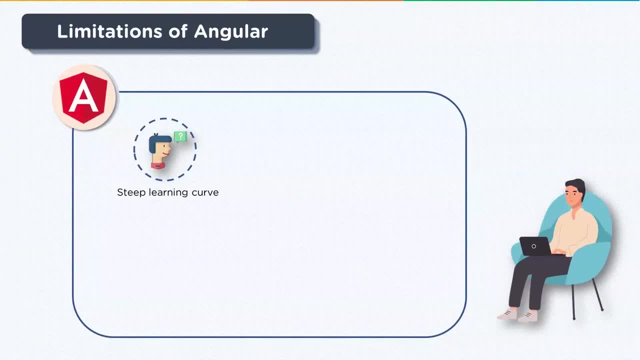 First up is a steep learning curve. Now, since Angular is a complete, full-fledged framework, it becomes difficult for learners. to begin with, You need to be acquainted with simple topics and then move on to more advanced topics to become proficient in this language. 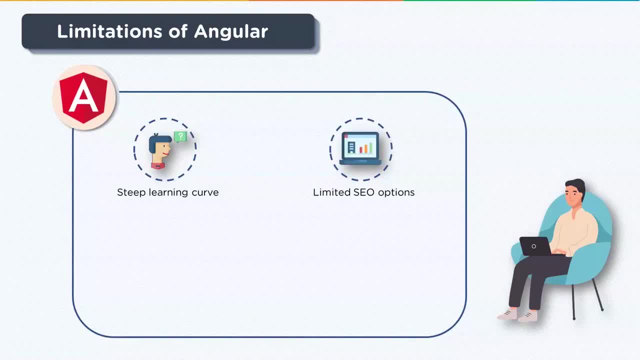 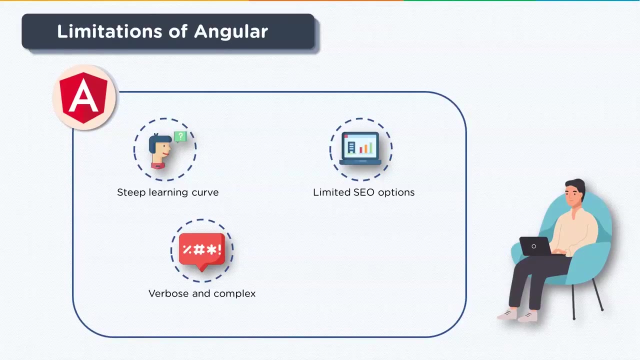 Next up is limited SEO options. Now, Angular offers limited SEO options and poor accessibility to search engine crawlers. It's verbose and complex. Now, a common issue faced by the Angular community is the verbosity of the framework. It also poses to be complex compared to other front-end tools.